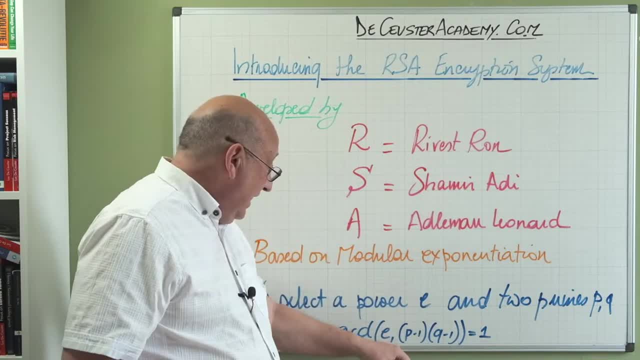 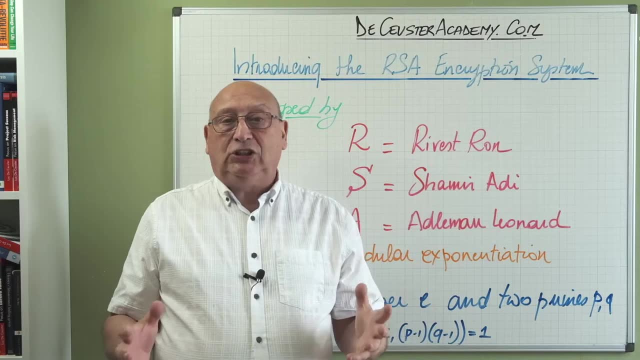 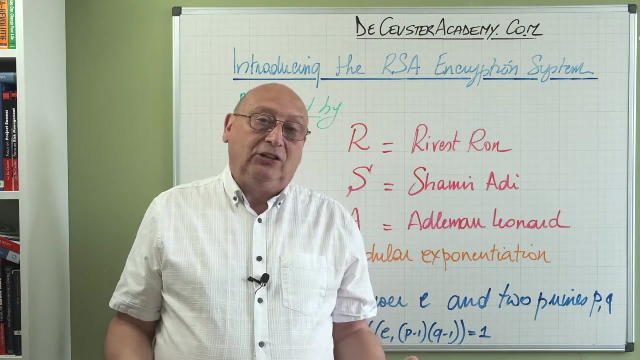 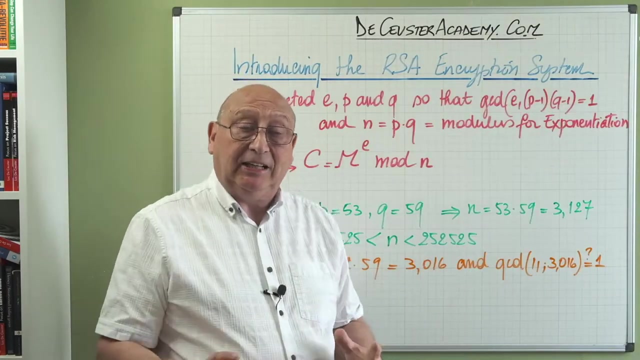 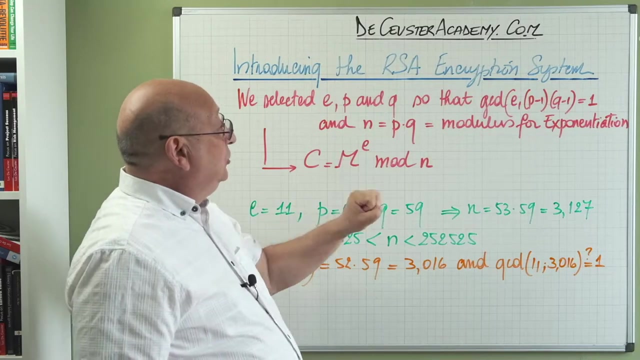 That e and the product of those two numbers are relatively prime Tes. have a look at how this system works using RSA encryption system. The NSsum encryption system starts with selecting the exponent and two primes, p and q, in such a way that the gcd of e and the product of p minus 1. 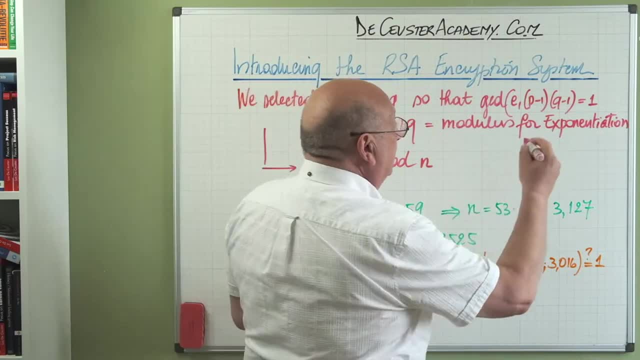 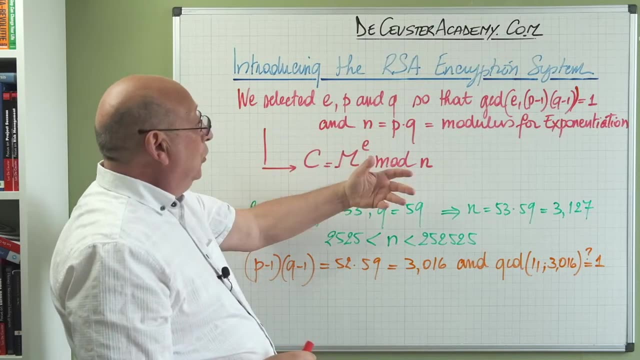 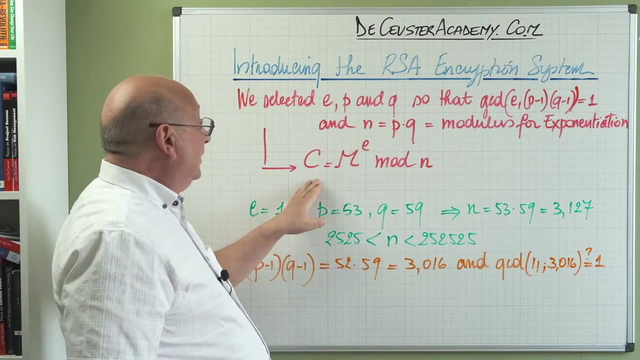 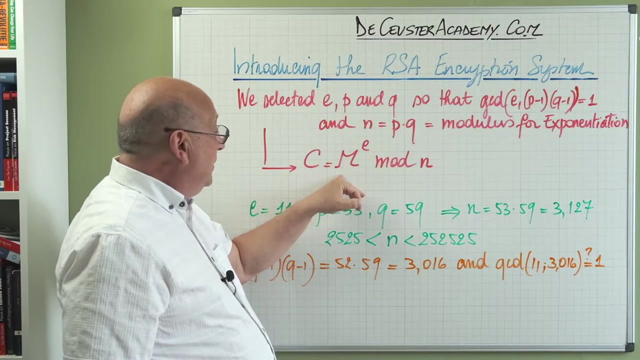 q minus 1 is equal to 1.. It means that those two numbers are relatively prime. Also, we have n, which is the modulus for the exponentiation, which is equal to the product of those two prime numbers, and the formula to encrypt any number. any text is. in fact, c is equal to m, to the power e modulus m. 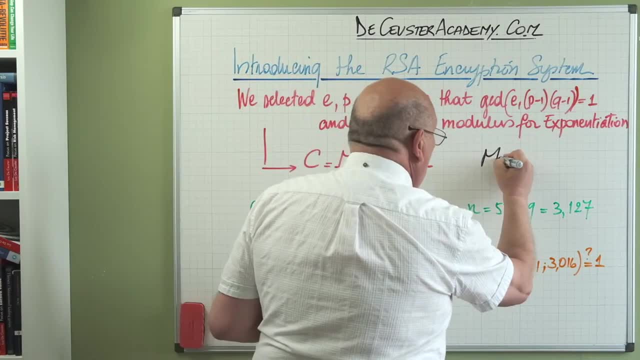 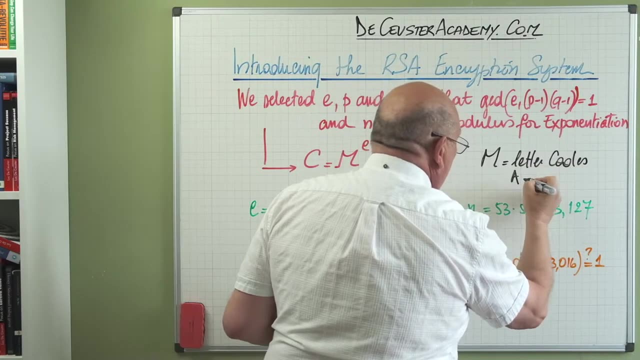 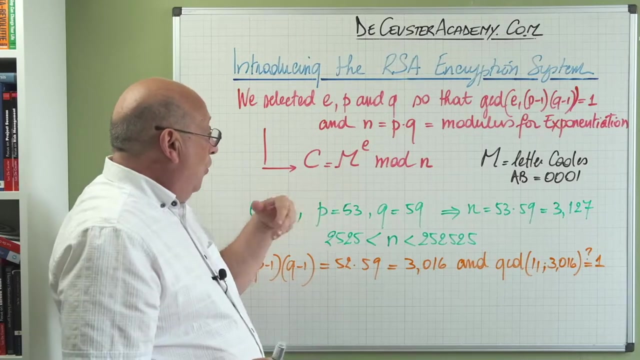 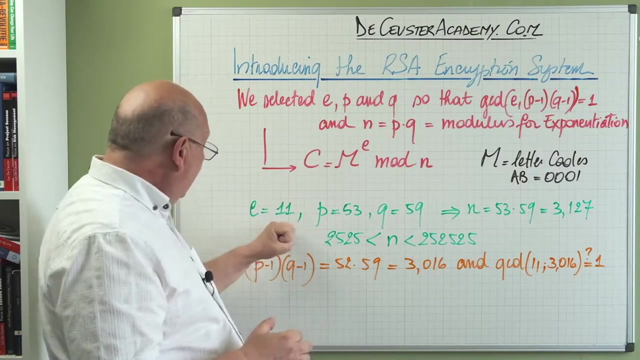 and m we obtain from the letter codes. for example, a, b would give me 0, 0, 0, 1, that would be m. Now what is important? First of all, we have to verify if those rules are valid. Let's say we selected for the exponent. 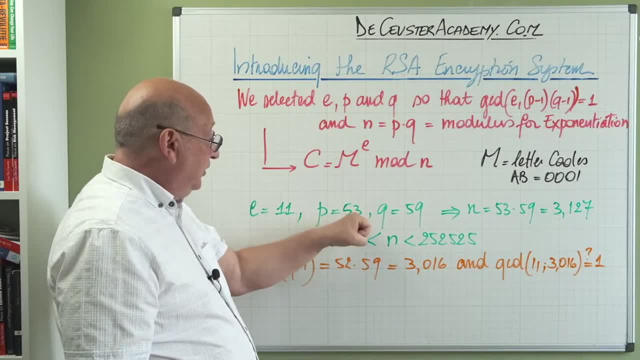 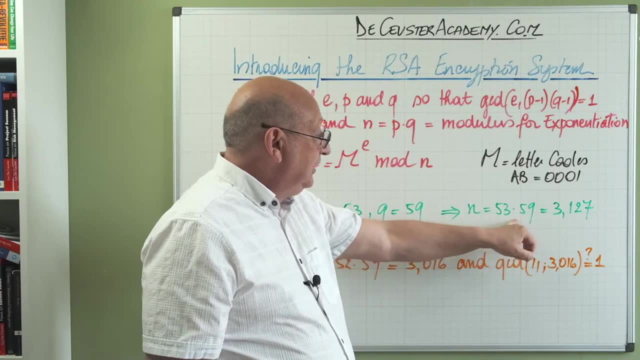 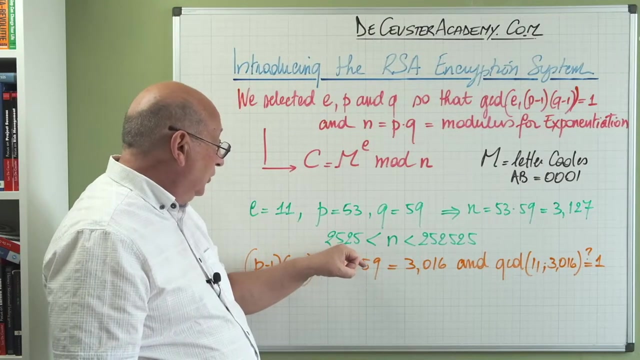 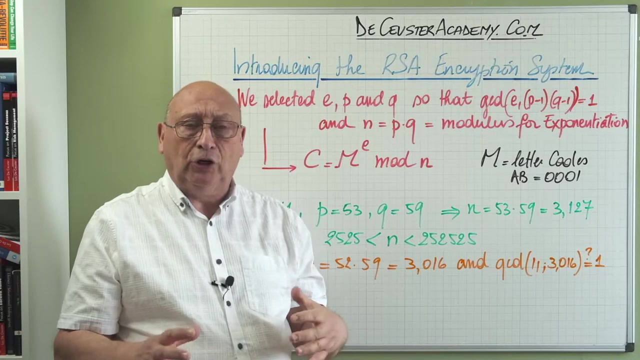 the number 11, p is 53, q is 59. both are prime numbers and we can calculate n, which is 53 times 59, which gives us 3127, and n is between 2525 and 253.. That relates to the system that those gentlemen developed. 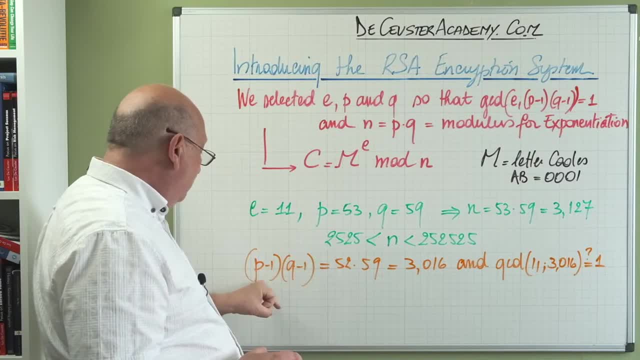 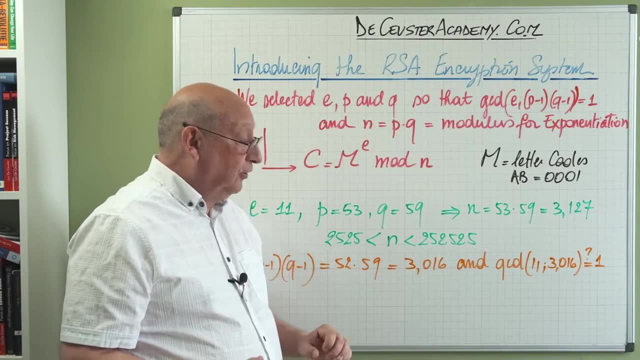 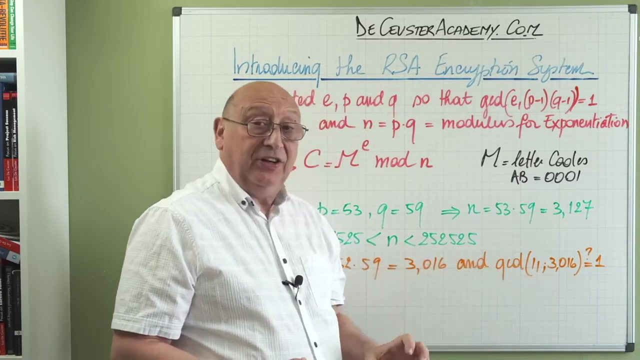 So, basically, what we now have to do is to calculate p minus 1 times q minus 1, which is 52 times 59, and it gives us a result of 3016.. Now we have to see if 3016 and 11 are relatively prime. 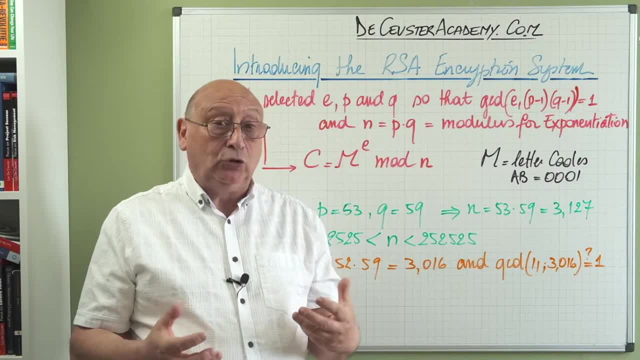 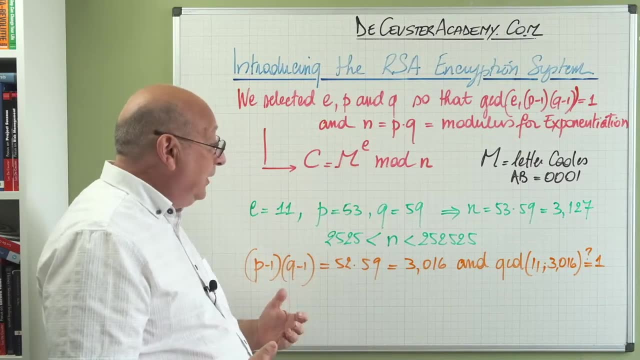 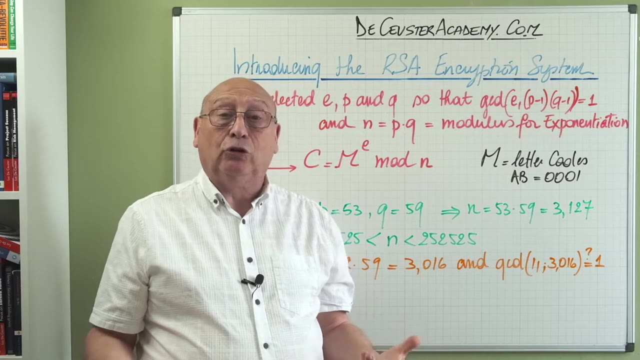 Why is this important? Well, in order to evaluate this, we have to calculate the value of the prime numbers in the star decrypt, a message. we have to do the inverse calculation and we have to find the inverse of e modulus 3,016, 11 modulus 3,016. that's only valid when 11. 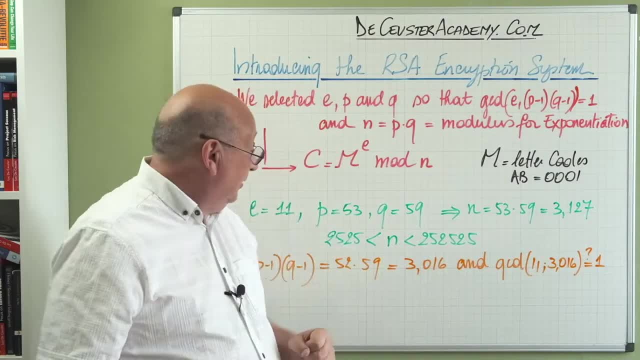 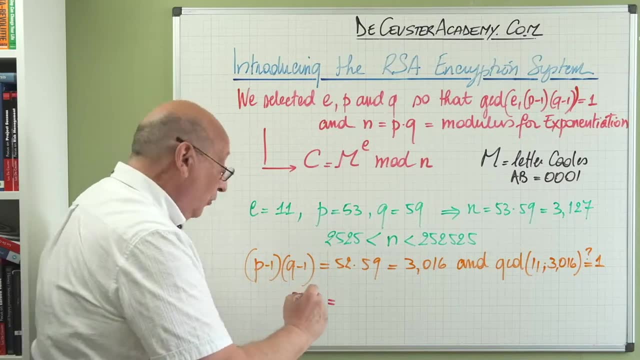 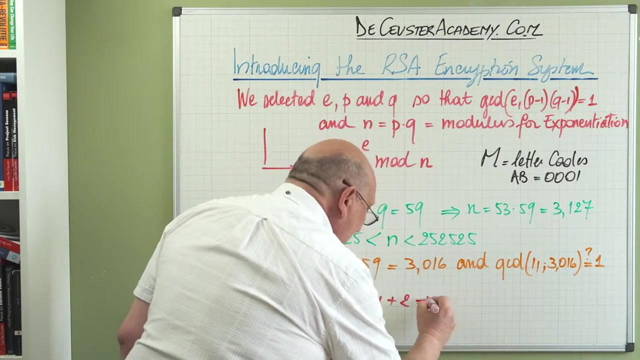 and 3,016 are relatively prime. let's have a look at that if it is true. so I can say that 3,016 is 274 times 11 plus 2, so we can say that 11 is 5 times 2 plus. 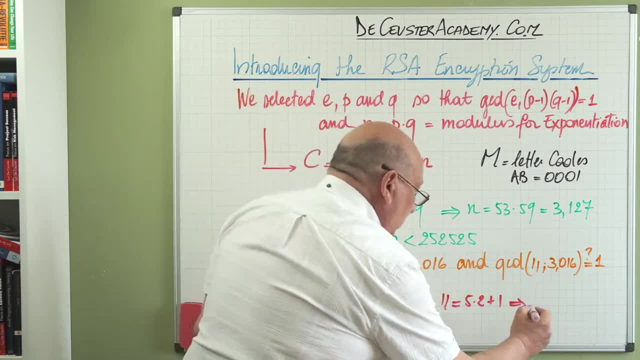 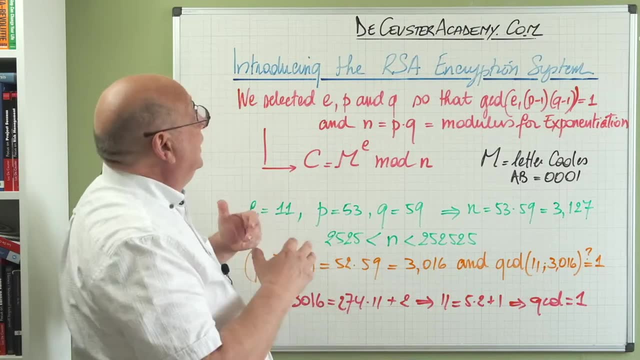 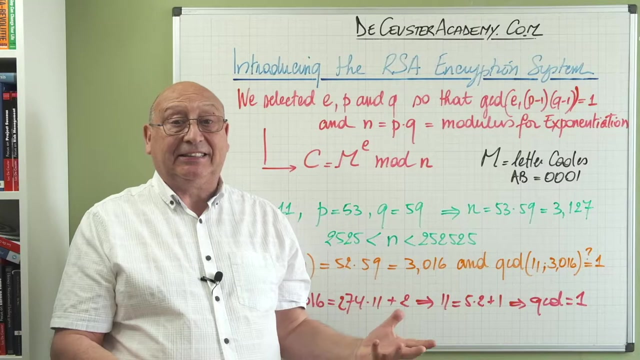 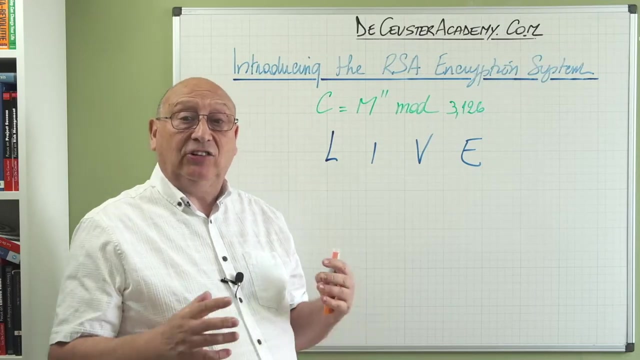 1, which means that the GCD is equal to 1. so, basically, we can use the NSA encryption system to with these numbers, and that's what we are going to do in the next step, based on the definitions and the selections we made before we can rewrite the 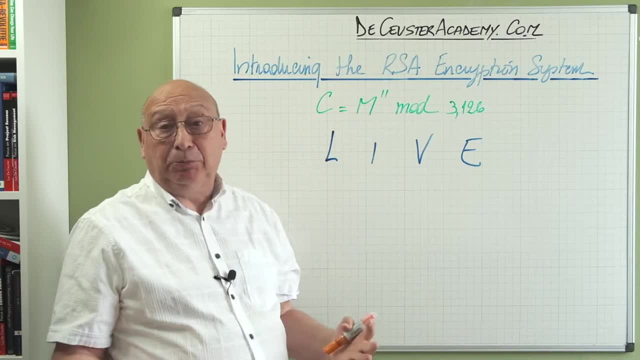 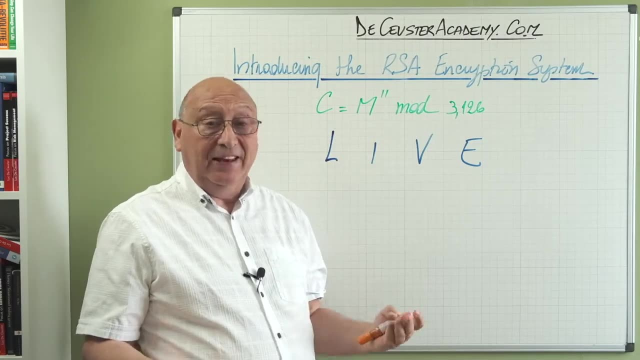 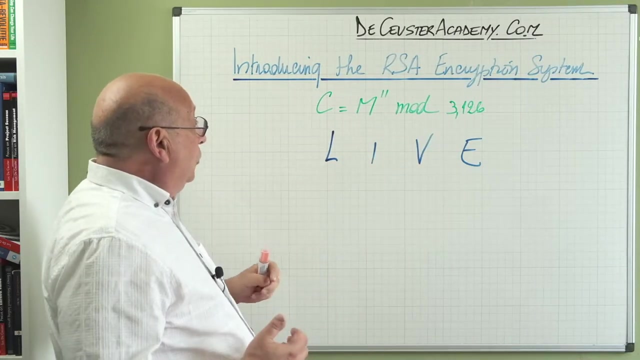 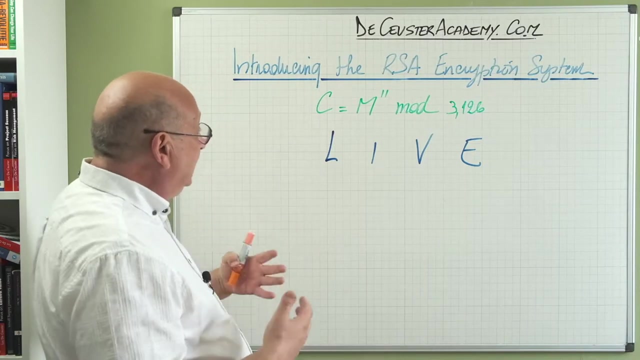 encryption formula, which is C, the encryption, the encrypted number that we will receive is M, the number two, and encrypt to the power 11, modulus 3,126. now, the word we're going to encrypt is the word life. so the first thing we do is to replace these numbers. 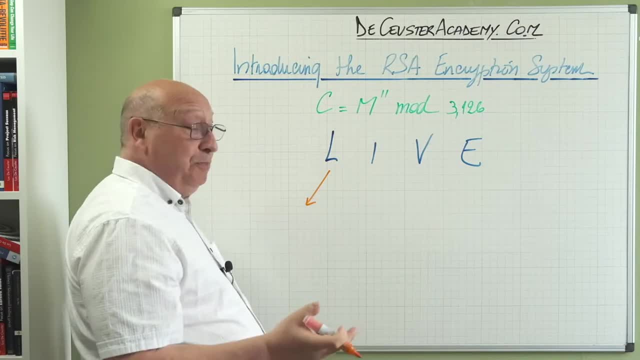 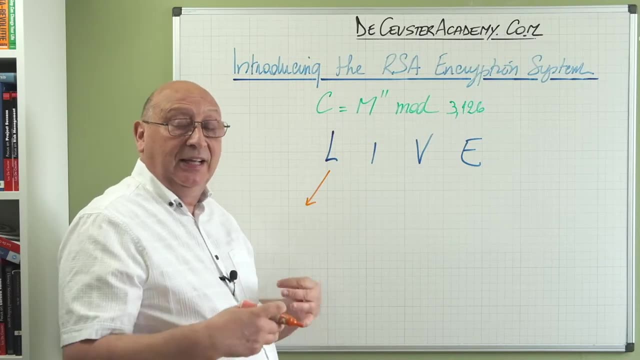 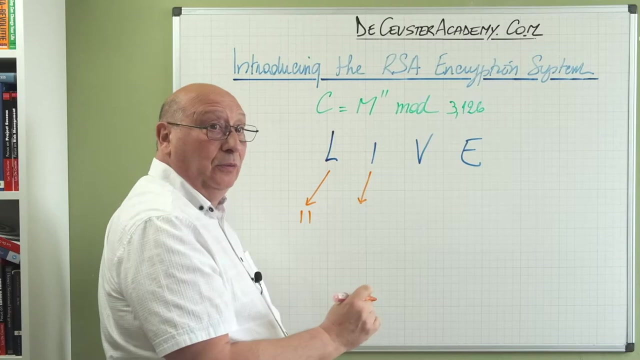 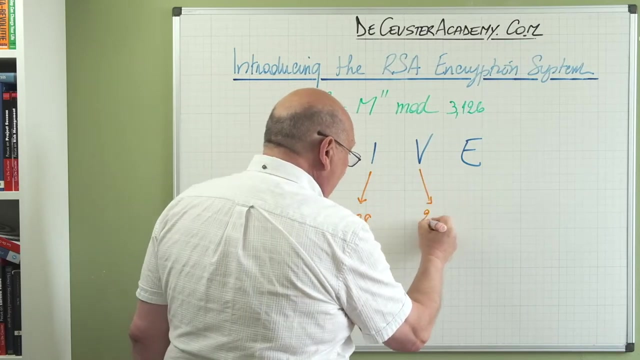 of these letters by a number. we did that before. we use the classical 26 letter alphabet, all in capital letters, no difference between capital and small letters. so it gives us 11, 4, l. we have i, which gives us 0, 8. we always use the two numbers: v is 21 and c is 0, 4. so basically we 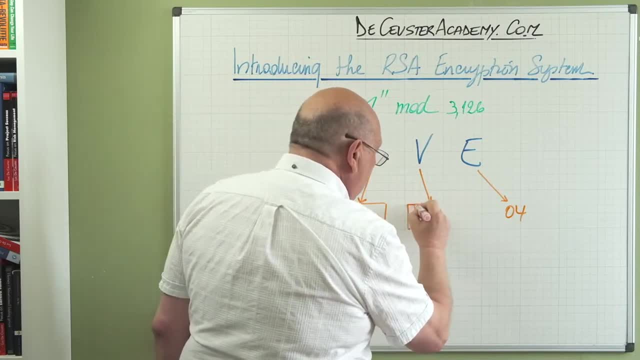 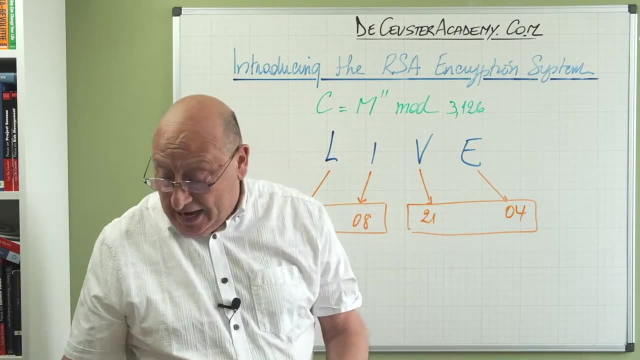 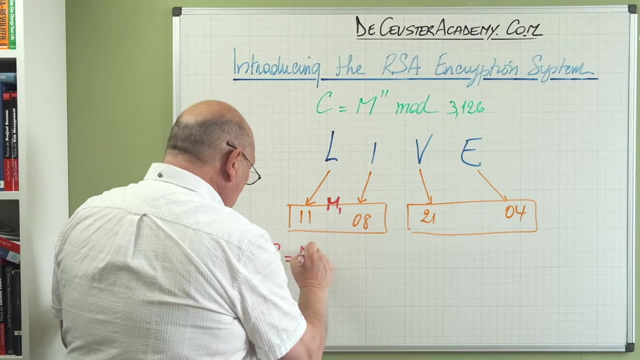 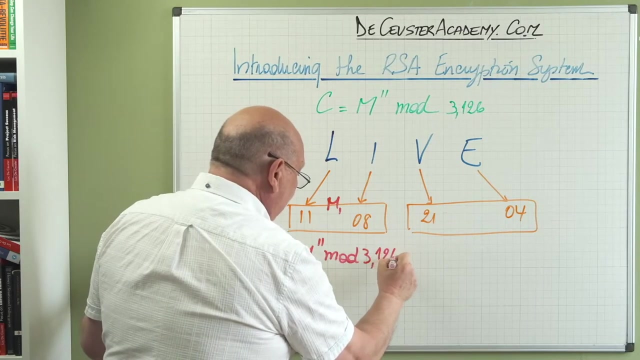 have two numbers here to encrypt, which are 11 0 0 8 and 21 0 4, and now we are going to apply the formula. so let's call this m 1 and we find c 1 is m 1 to the power 11, modulus 3126, and you can do that in different ways. you can. 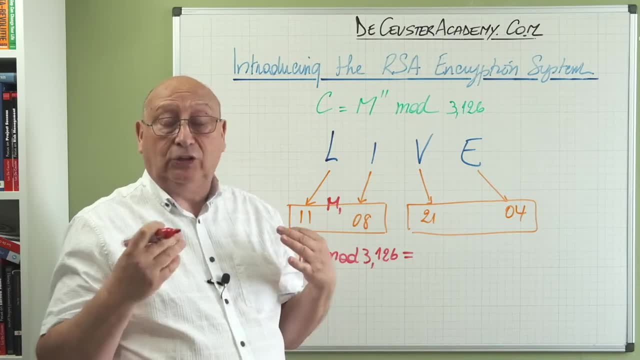 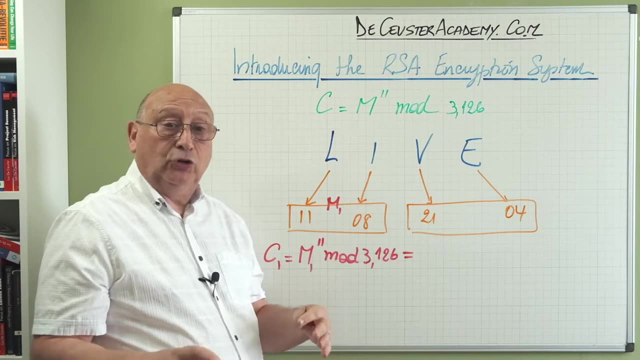 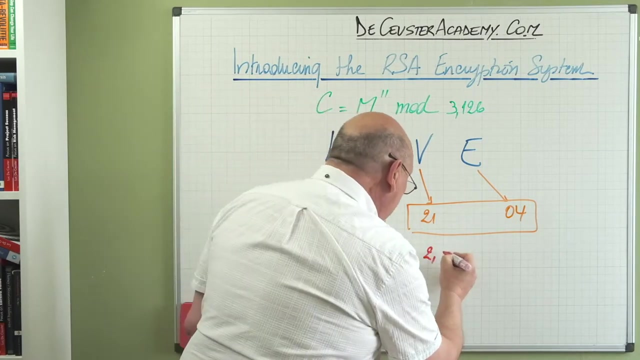 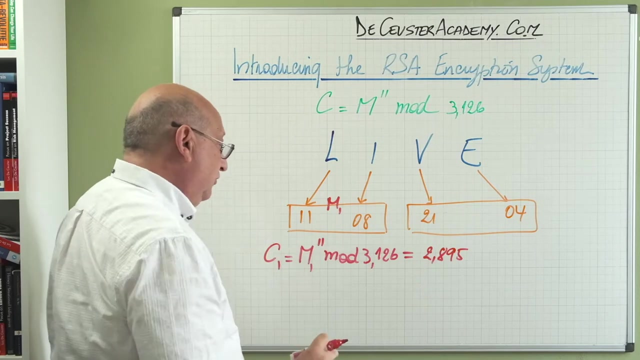 use a website to do this. you can use the modular exponentiation. that can be done anyway. i did the calculation for you- you can verify this for yourself- and we find that is two thousand 800 n and i have to verify 95. so basically that's the first number. we can take out the 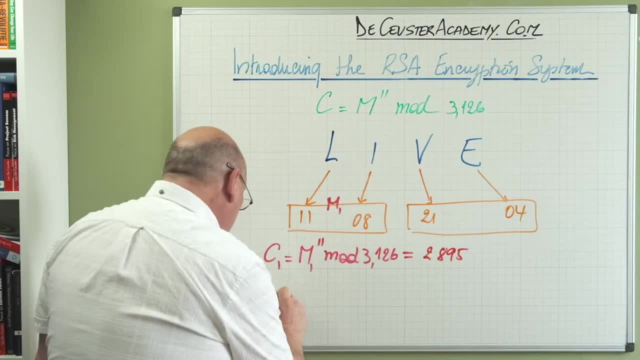 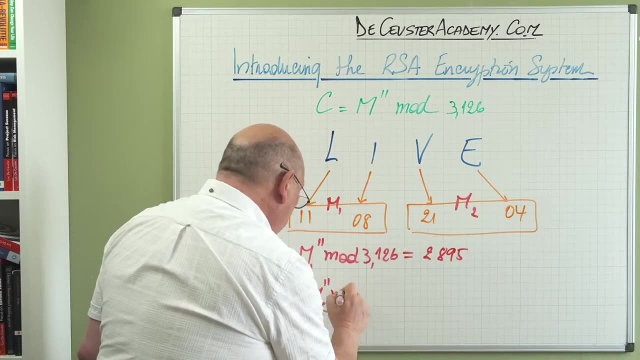 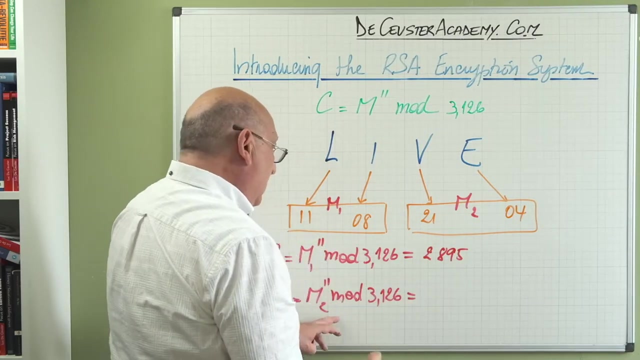 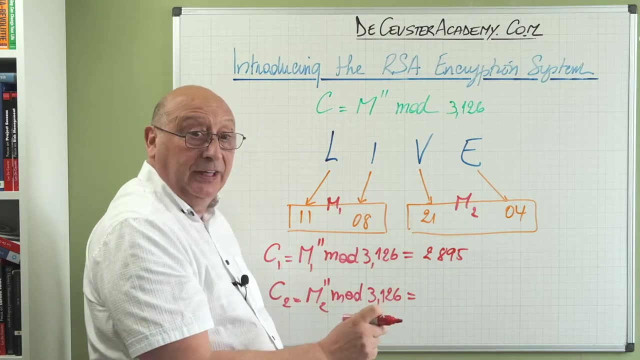 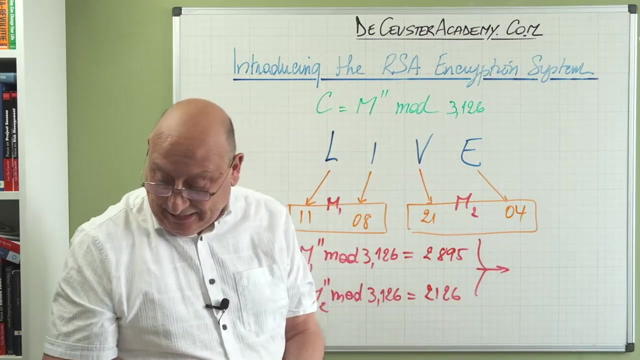 comma, because this has no sense here anymore. c2 is m2, which is this code here. to the power 11, modulus 3126, and we find here that it's two thousand one hundred and four. to the power eleven, modulus three thousand one hundred and twenty six is in fact twenty one twenty six, and based on this we can say that the coded message 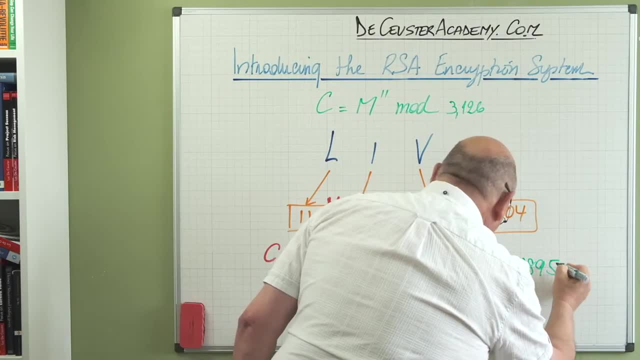 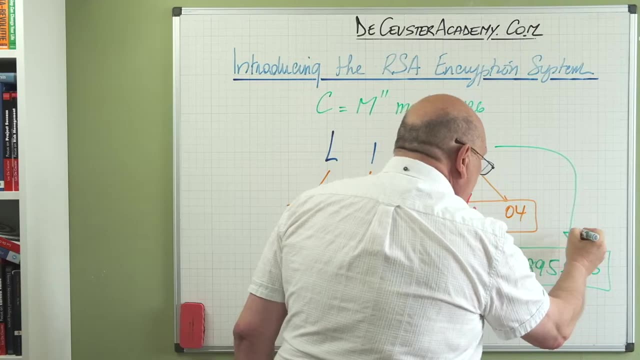 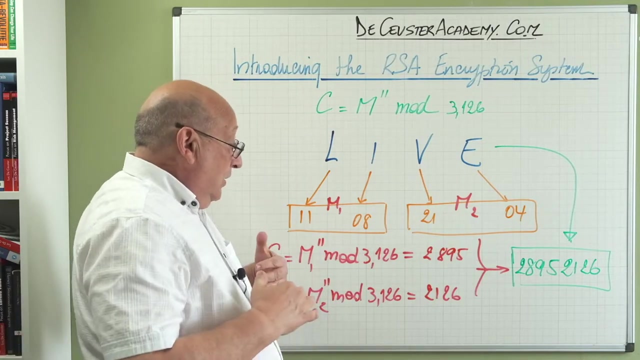 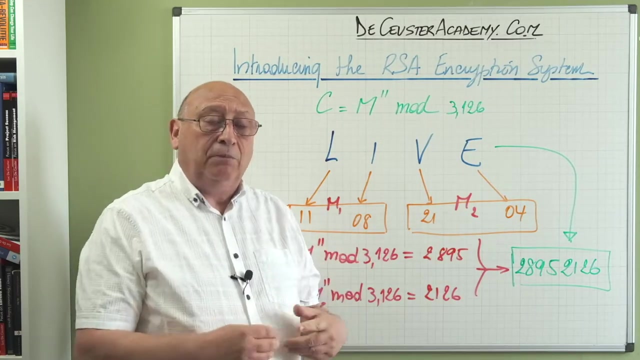 is two, eight, nine, five, two, one, two, six. so basically this has been coded into this series of numbers. this is almost impossible to crack. with these numbers that we have here, it's not so difficult. but when we use large prime numbers, when we use large powers, this becomes really. 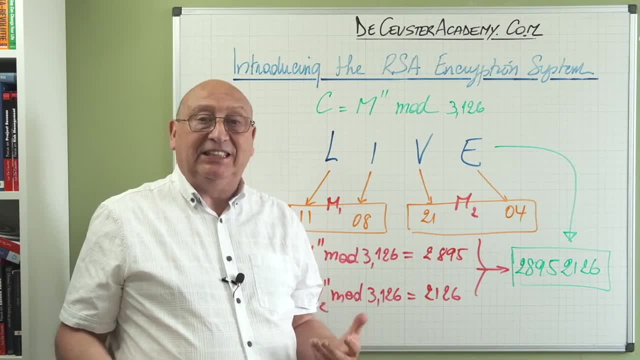 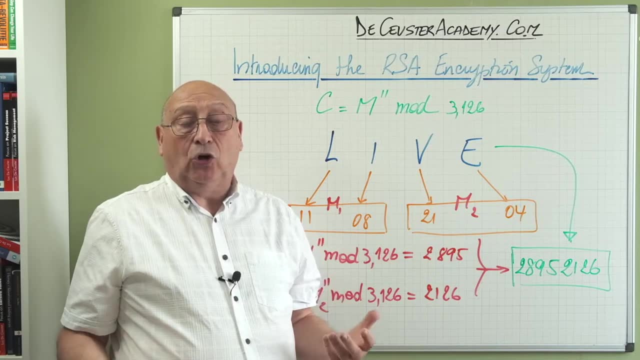 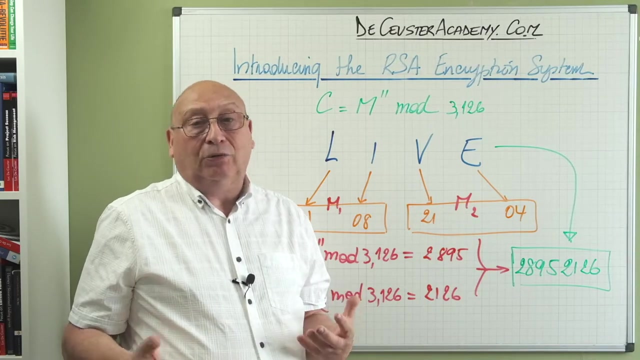 difficult to crack- basically impossible with the means that are available now. anyway, any code can be cracked, but the thing is that by the time a code will be cracked, it's not relevant anymore, and people change the keys from time to time, so you keep the security going, of course. today i've 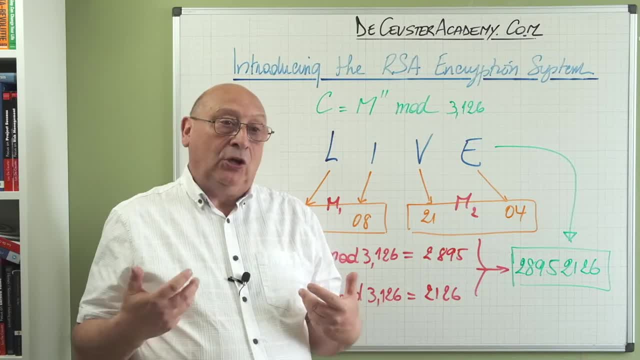 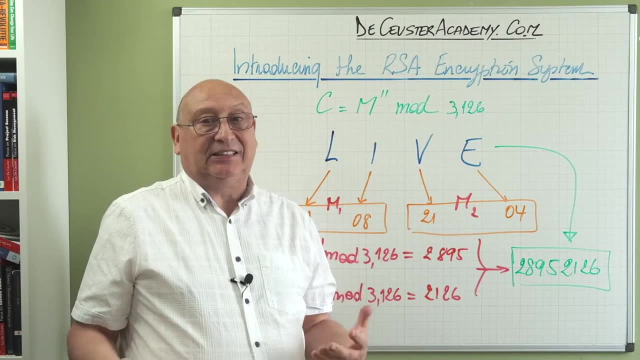 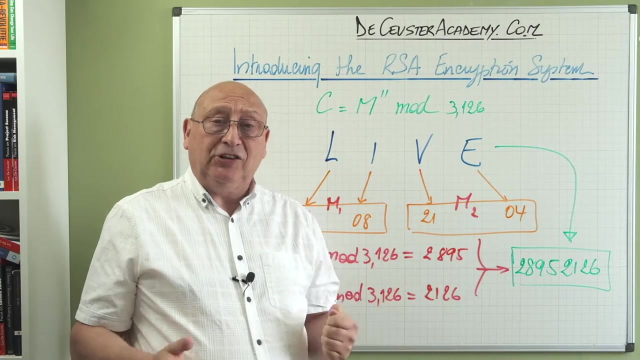 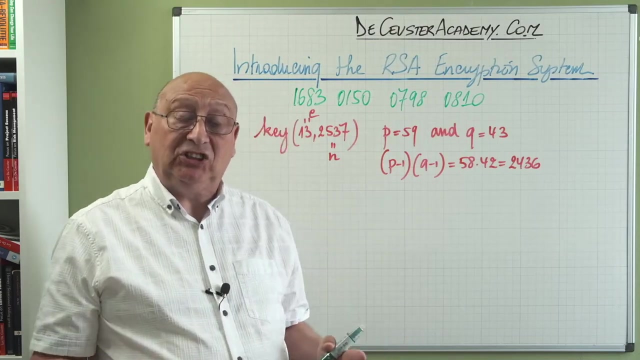 read some things about quantum computing and the expectation is that quantum computing can change things related to encryption, but we don't know for sure yet. we will see how the evolution will go. but let's now have a look how we can decrypt this message. let's now look at an encrypted message that we received, and the encrypted message is 1683. 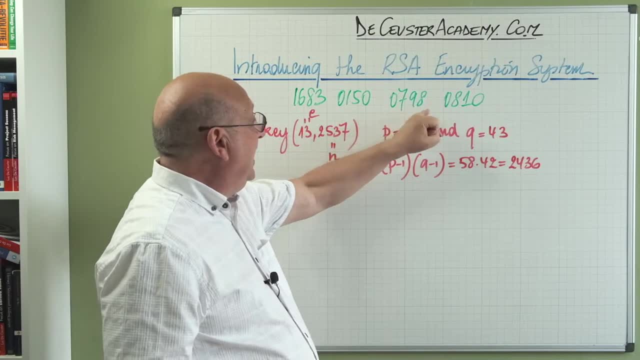 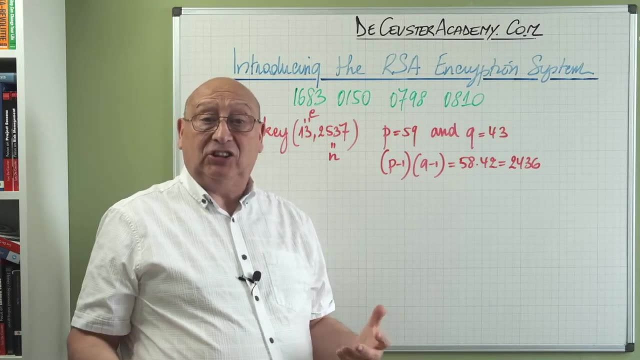 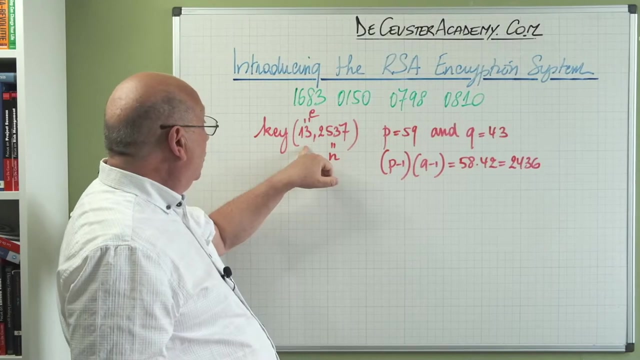 zero one five zero, zero seven. nine eight zero, eight one zero. basically, we want to know what was the real message, the clear message that was sent to us. now we know the key. we know that the key is 13, the exponent, and n, the product of the two. 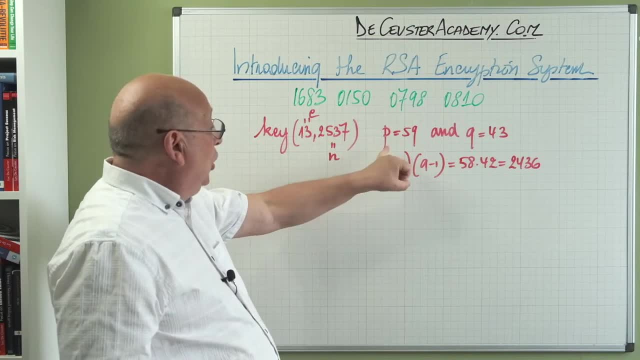 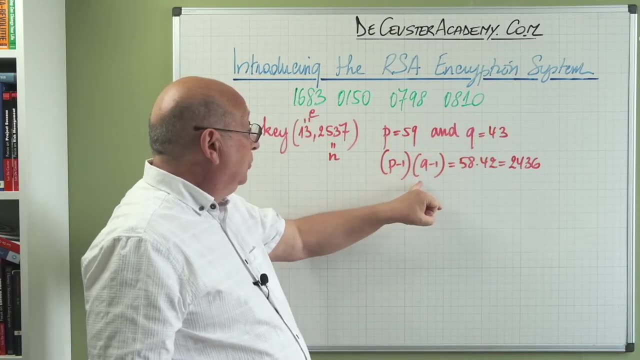 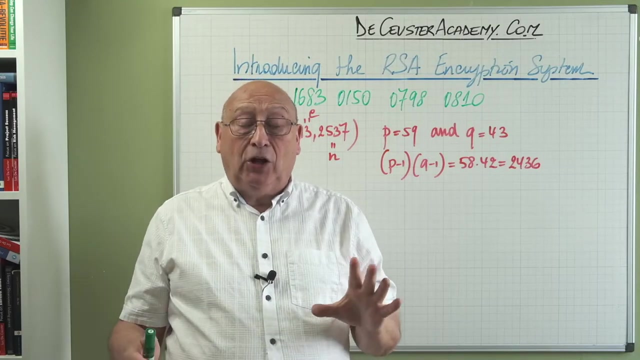 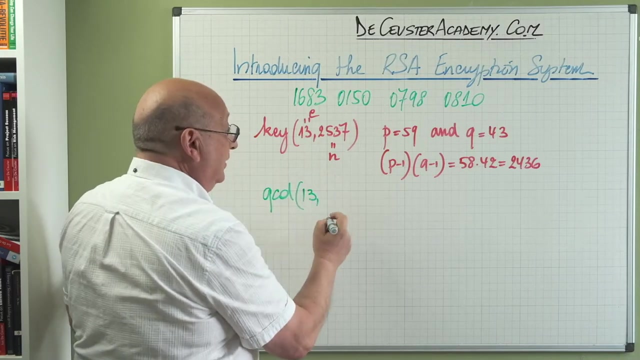 numbers 2537, with p equal to 59 and q equal to 43. we also know that p minus 1 times q minus 1 is 58 times 42, which is 2436. now the first thing to see is the gcd of 13 and 2436. is it equal to 1? 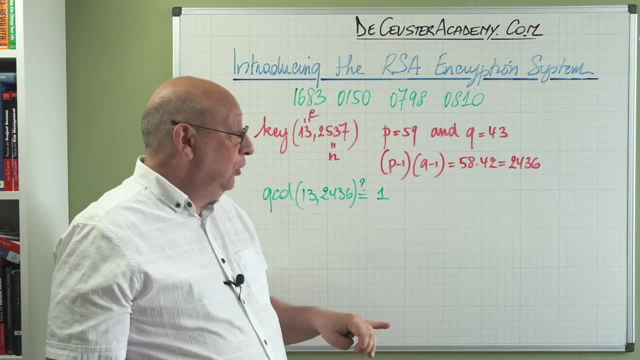 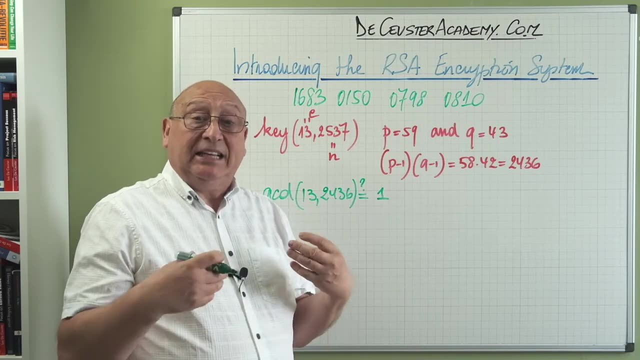 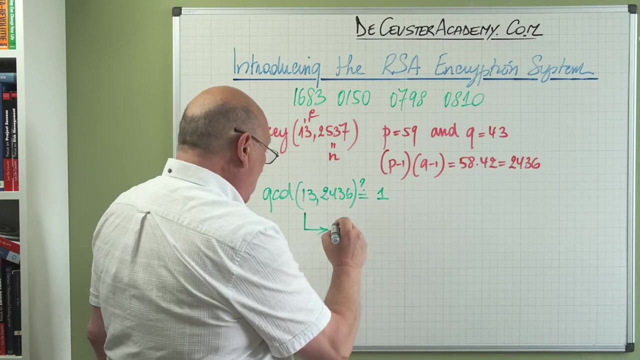 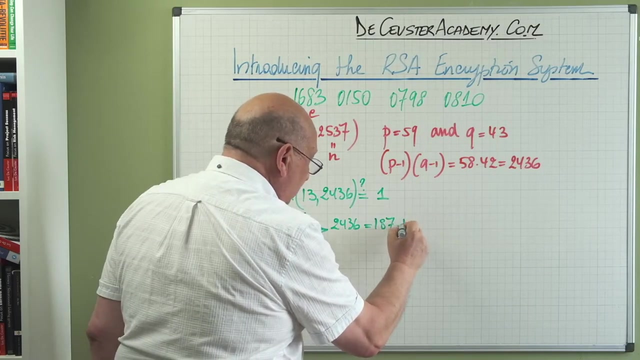 because we have to know the modular inverse of 13 modulus 2436 to be able to decrypt the message. Now let's have a look at this GCD So we can say that 2436 is equal to 187 times 13 plus 5.. 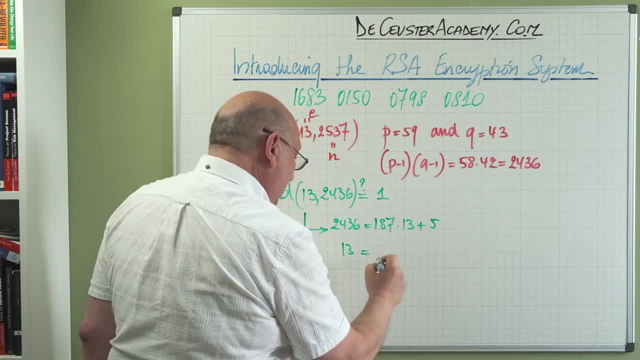 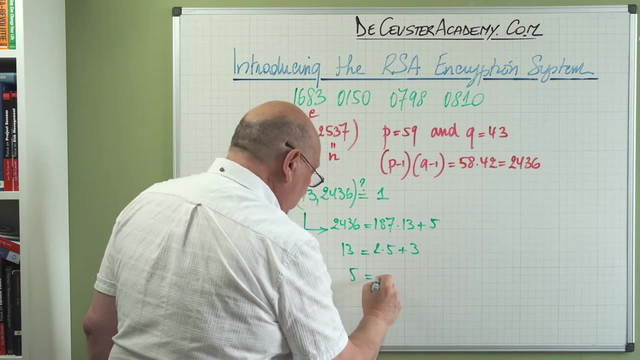 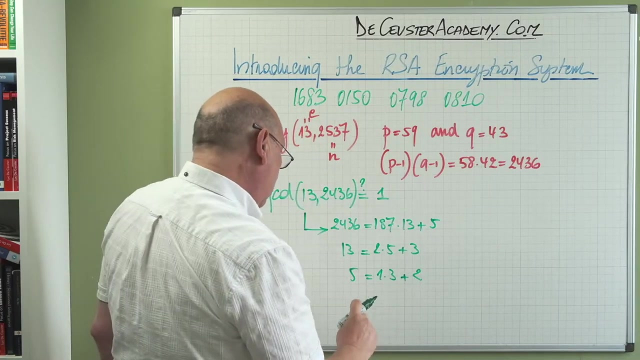 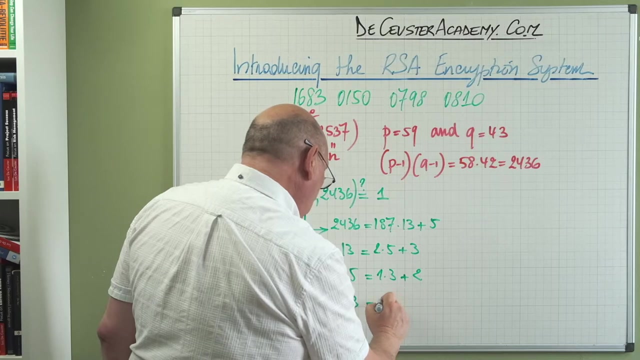 Now we can say that 13 is 2 times 5 plus 3, and 5 is 1 times 3 plus 2, and finally we find that we have 3 is 1 times 2 plus 1, which means that the GCD. 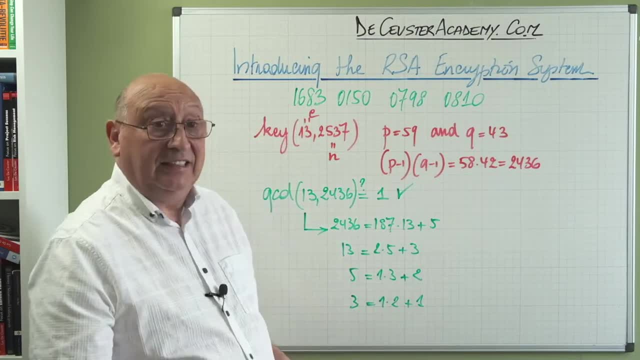 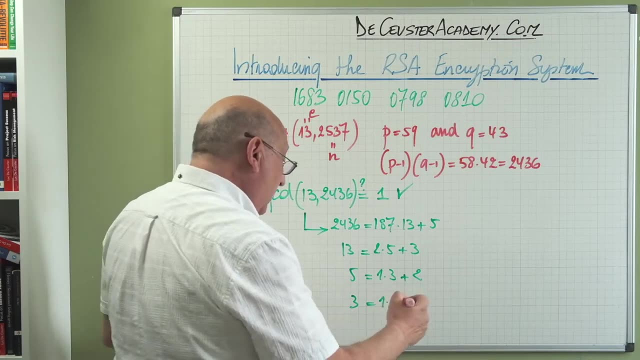 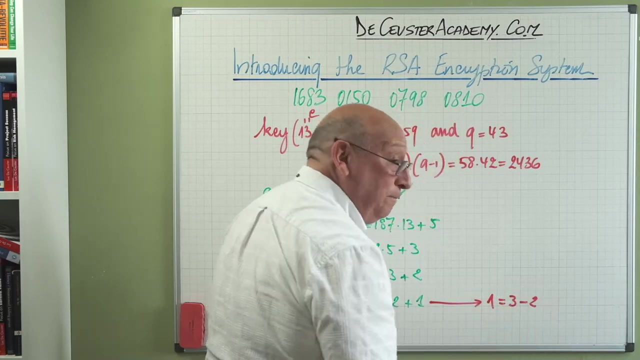 is equal to this. Now we have to calculate this in the other direction, We have to find the calculations in the other direction and we start from here. So we have: 1 is equal to 3 minus 2.. So we have 3 minus 2.. 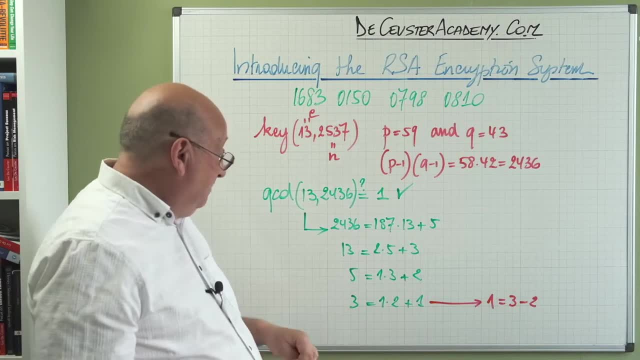 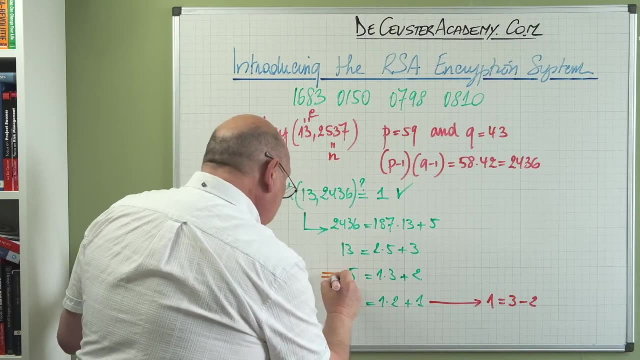 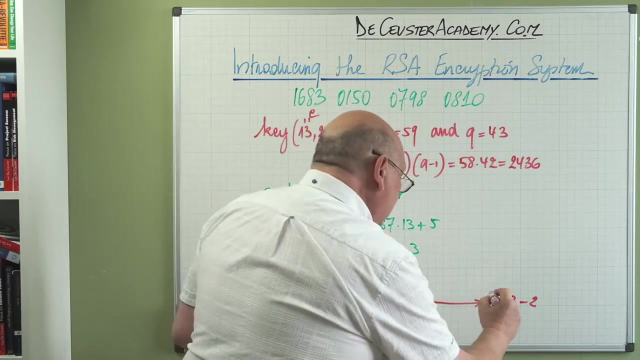 That's the first step that we have. Now we put 2 in there and we know- and I will put it on this side- We know That 2 is equal to 5 minus 3.. So when we put it in here, 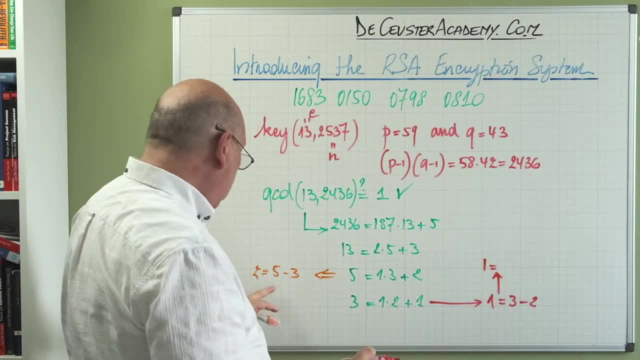 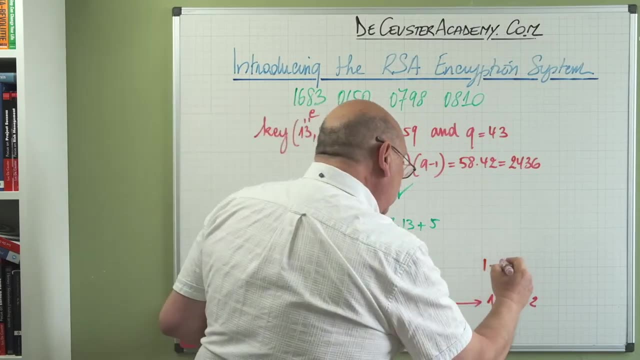 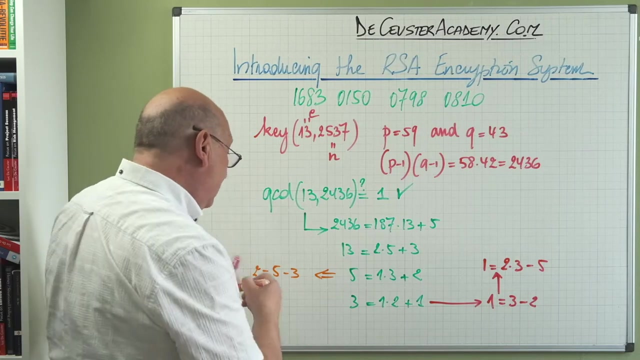 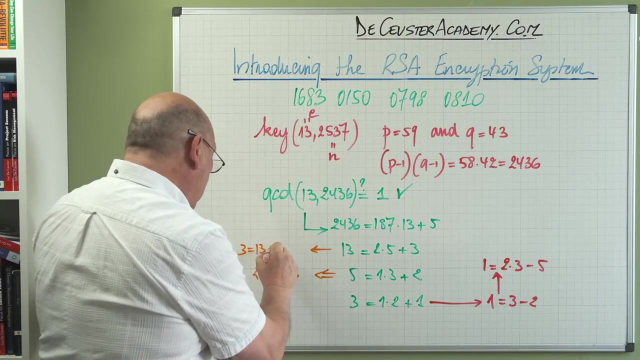 We can say that 1 is equal to 3 minus 5 minus 3.. So we have 2 times 3 minus 5.. Which is still correct. We can verify that easily. Now we have to replace 3.. And 3 is equal to 13 minus 2 times 5.. 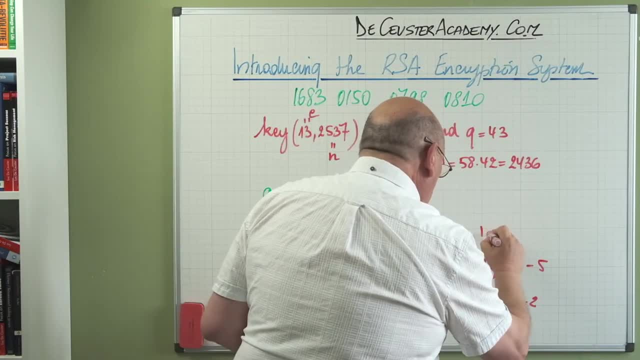 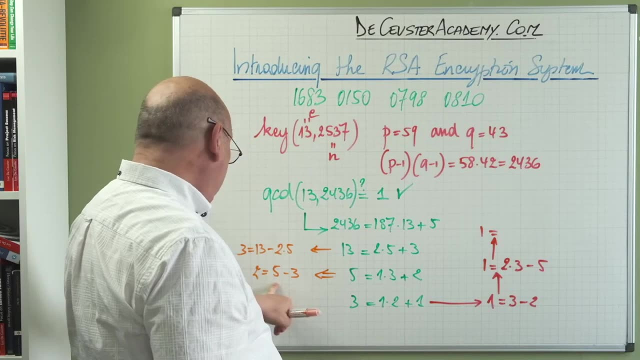 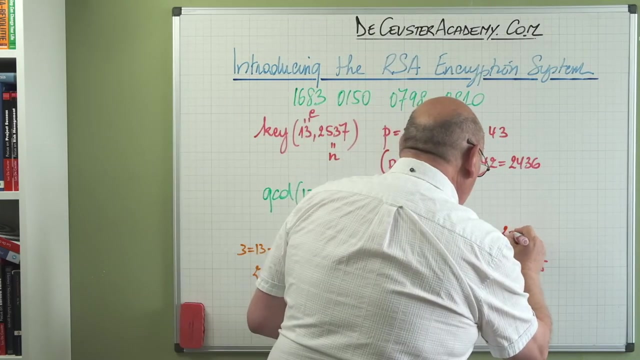 We bring that value in here again, So we say 1. We have 2.. So we have 3 times 5.. Sorry, We bring 2 in here, So we have 2 times 13.. 2 times 13 minus 4 times 5.. 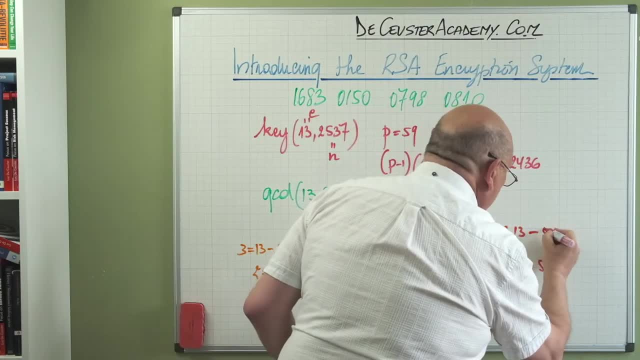 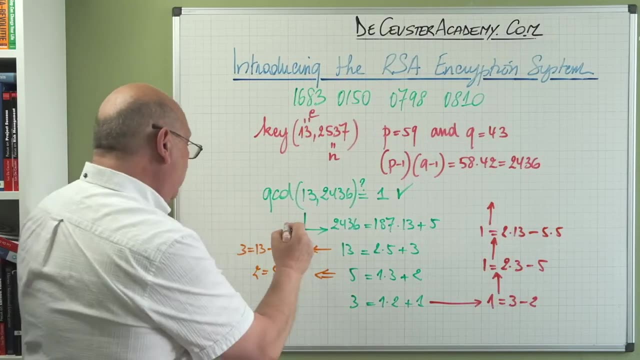 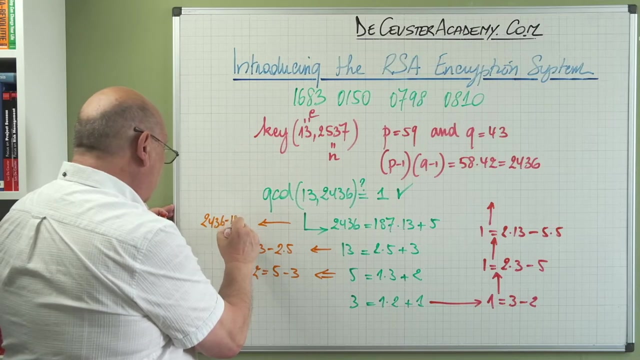 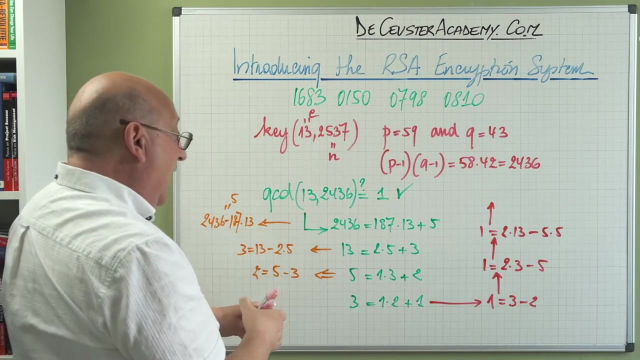 5 minus 5.. 5 times 5.. And the last step, where we will find the inverse. We use this last formula. We can say that 2436 minus 18 times 7 times 13 is 5.. So basically, I replace 5 in here. 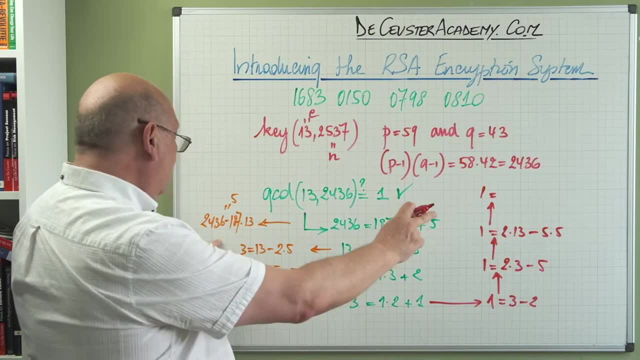 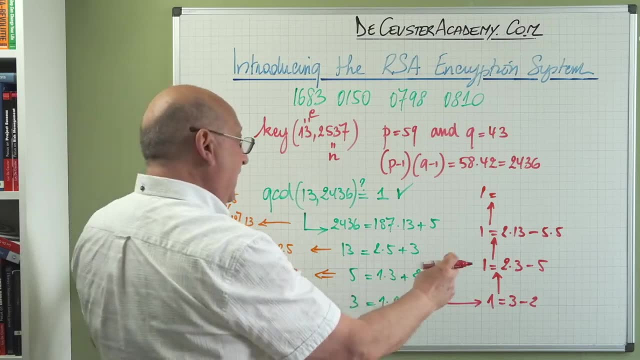 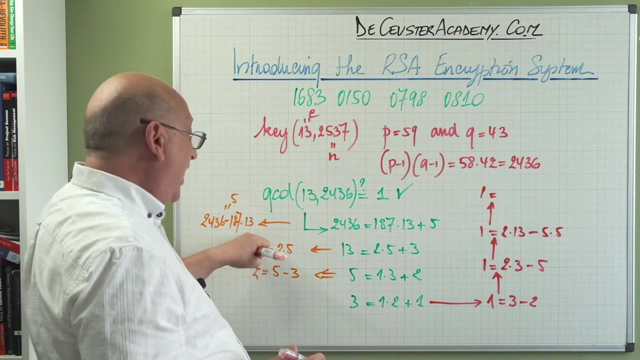 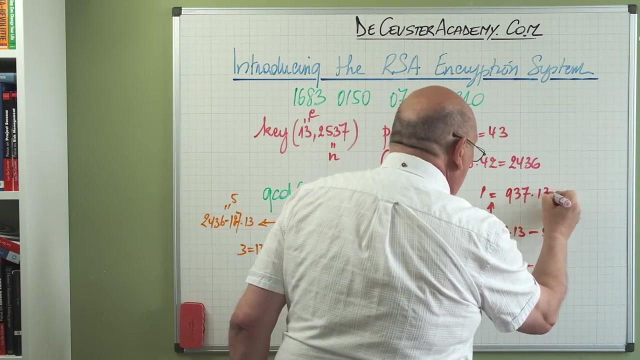 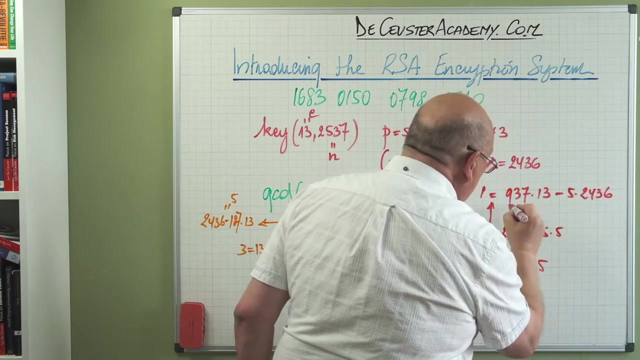 So we have 2 times 13.. Minus 5 times 5.. So I have 187 here 5 times 187.. Which is 935.. Plus 2. 937 times 13.. Minus 5 times 2436.. 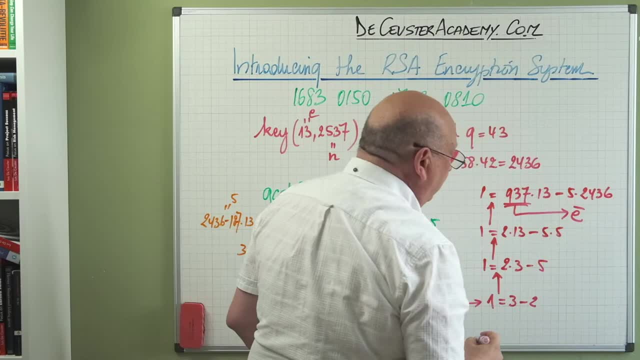 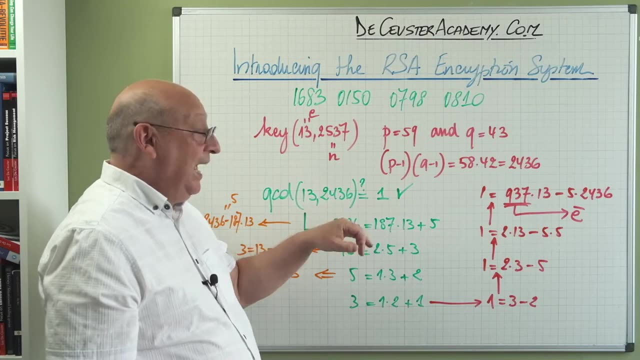 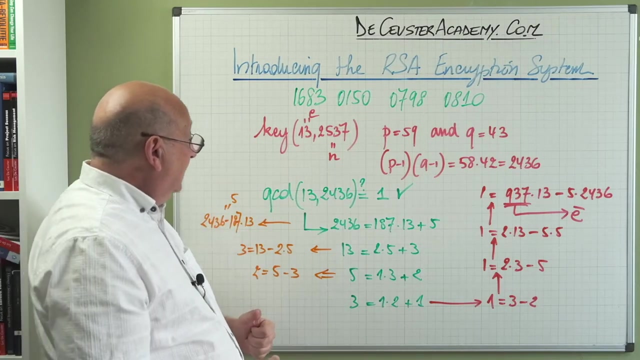 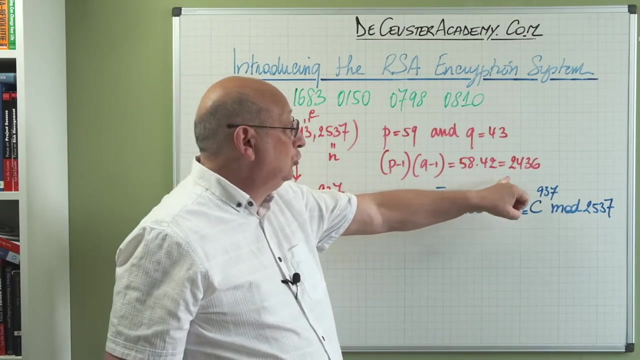 And this number is the inverse of E, modulus 2436.. And that's what we are going to use to decrypt the message. Let's do that. when I clean this board, We found the modular inverse of 13, modulus 2436.. Which is, in fact, 937.. 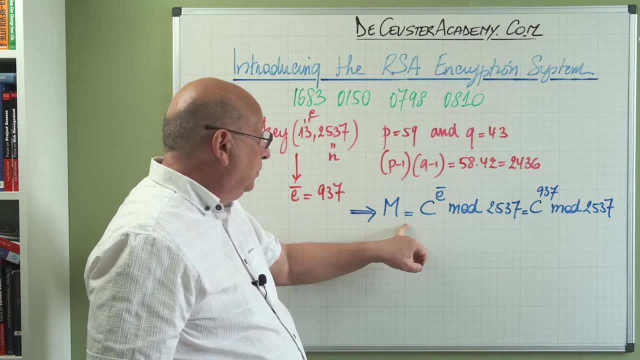 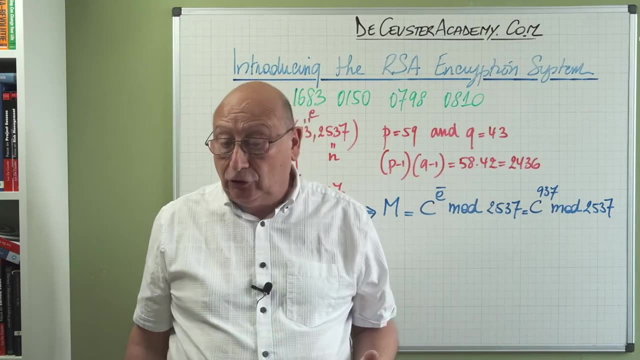 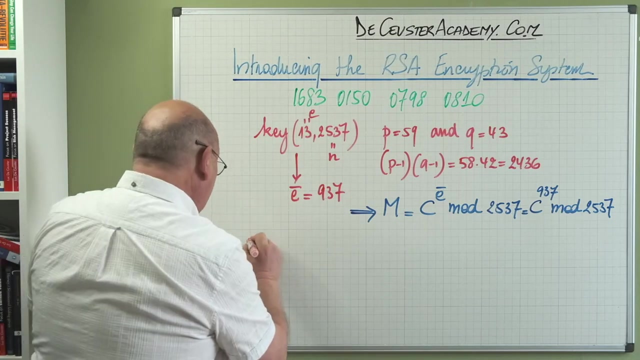 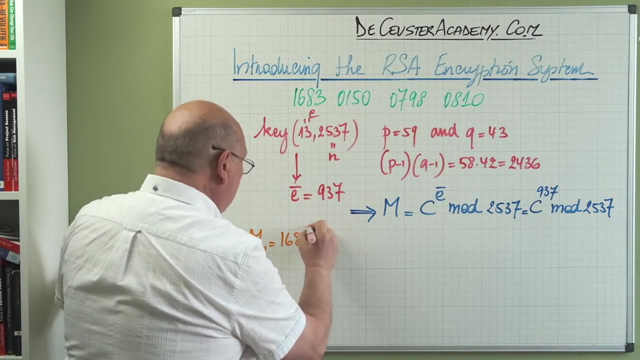 Which gives us the decryption formula to be equal to C to the power of 937, modulus 2537.. What we remain to do is to decrypt this number. So basically we can say that M1, the first set of 4 letters, is 16A3 to the power 937. 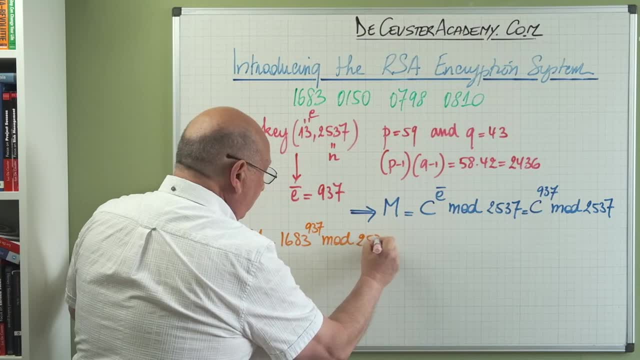 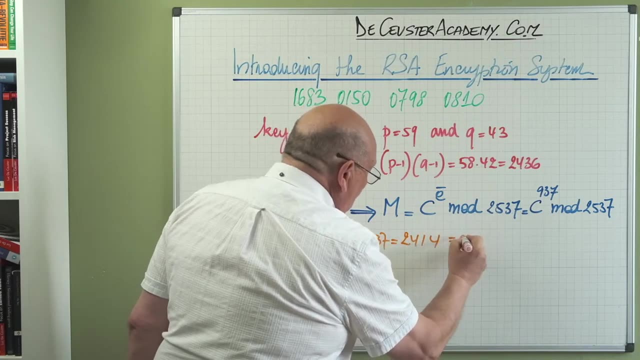 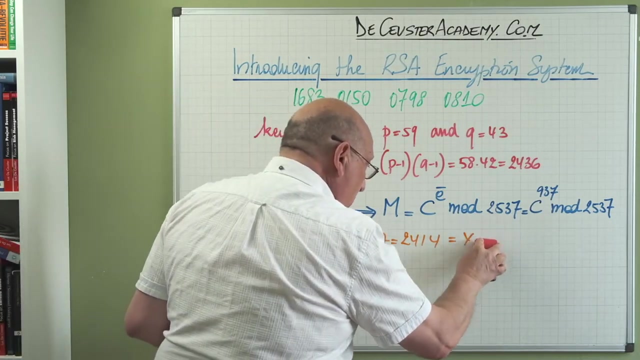 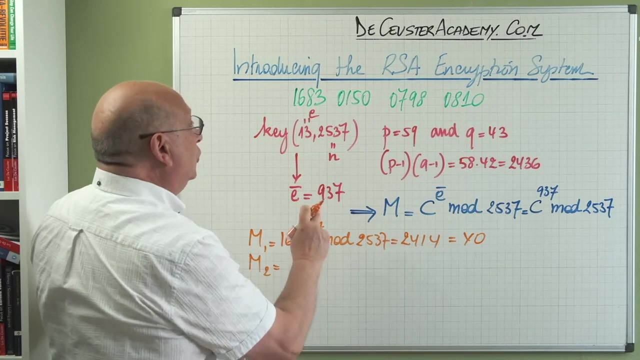 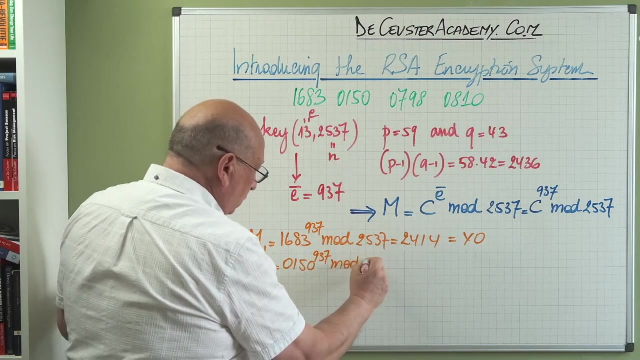 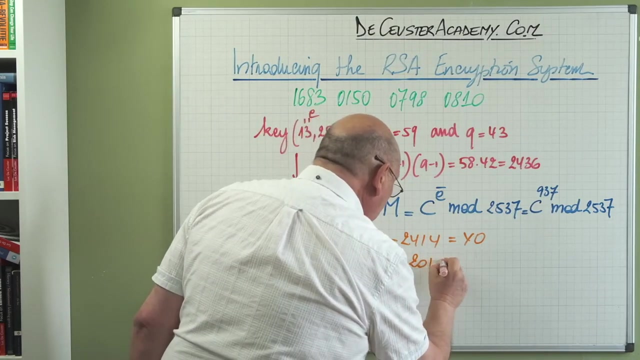 Modulus 2537. Which gets you 2440.. Which is Y and U, Sorry O. Then we have M2., Which is equal to 0150.. To the power 937.. Modulus 2537. Which gives us 2019.. 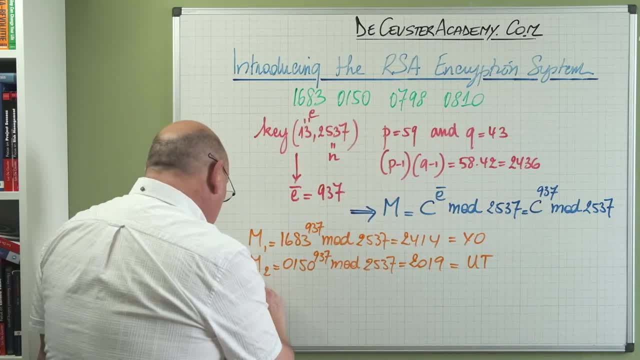 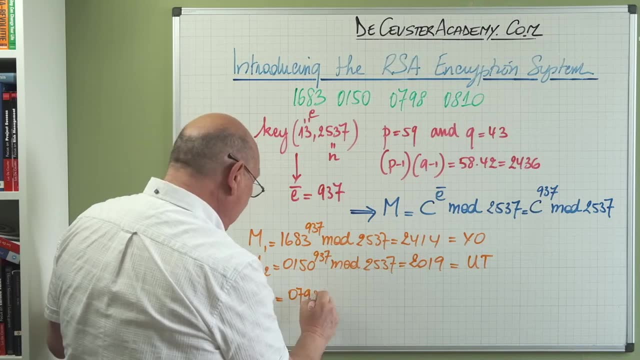 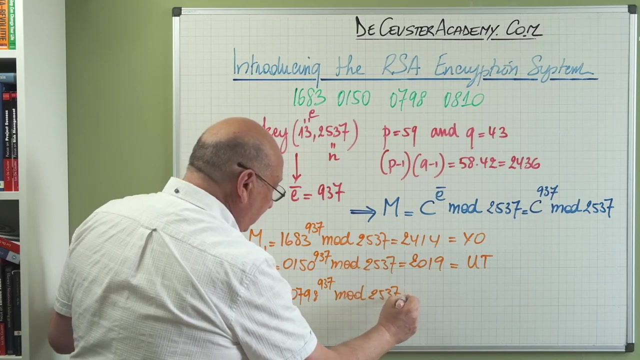 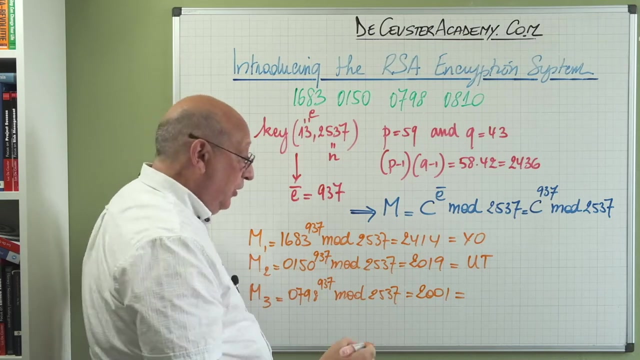 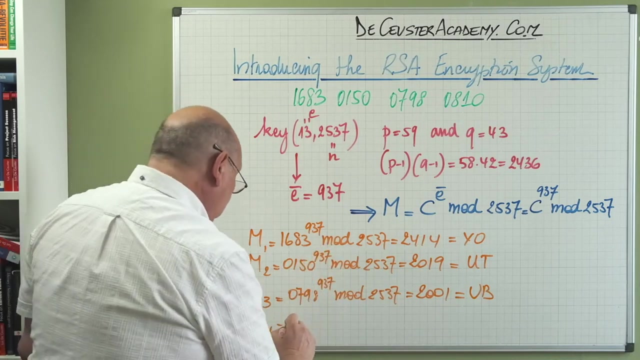 Which is U and T, Then we have M3.. The third one is 0798 to the power of 937.. Modulus 2537. And that gives us 2001.. And it gives us the letters U and B, And M4 is 0810 to the power 937. 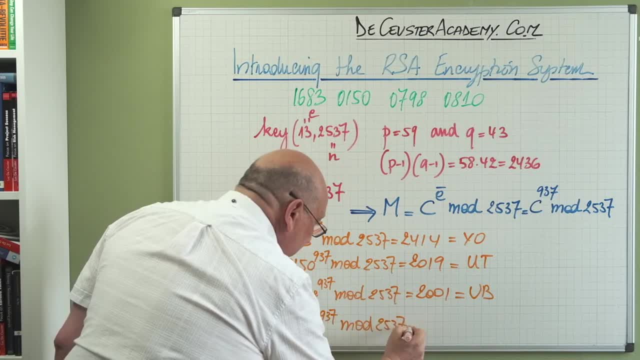 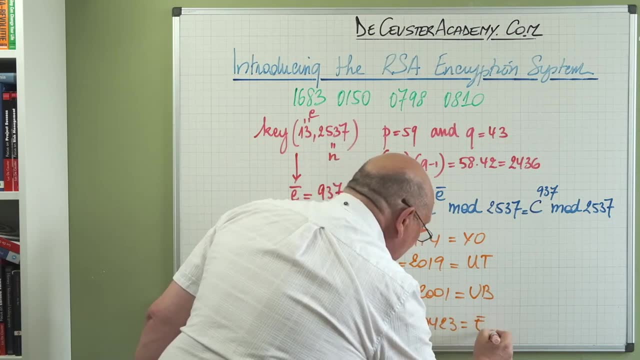 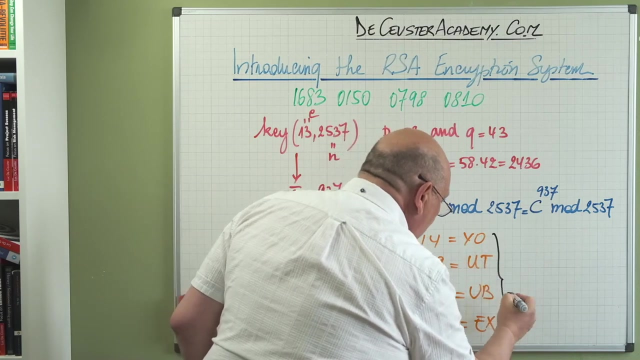 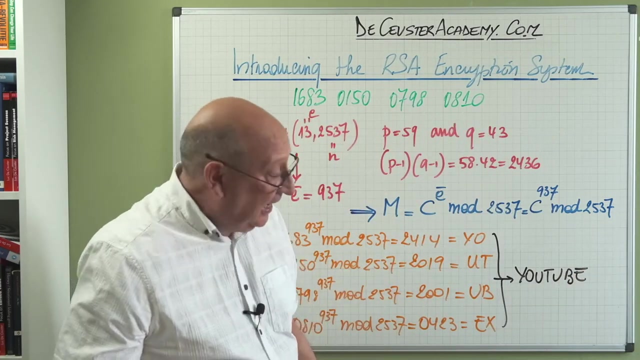 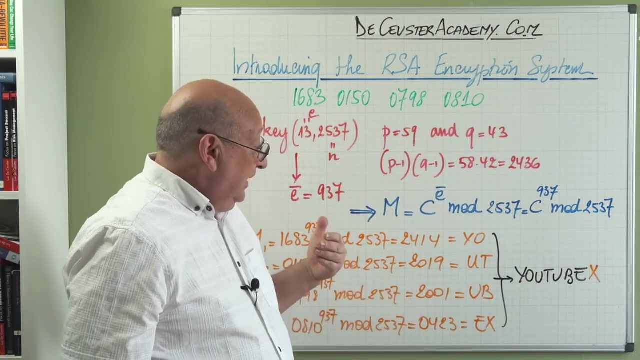 Modulus 2537. Which gives us 0423.. Which is E and X. Now when we look at this and we write this message again, We find that is U tube And there is an X at the end. An X we added just to see that we have basically numbers, which represents two characters. 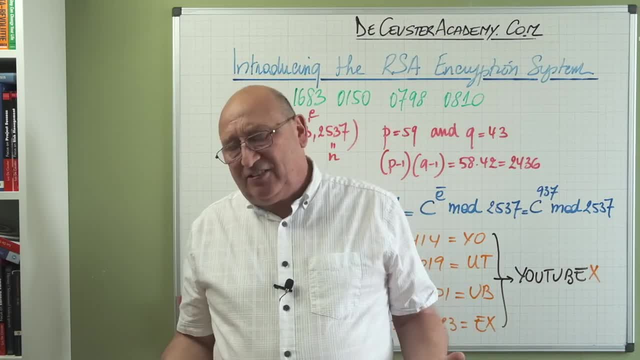 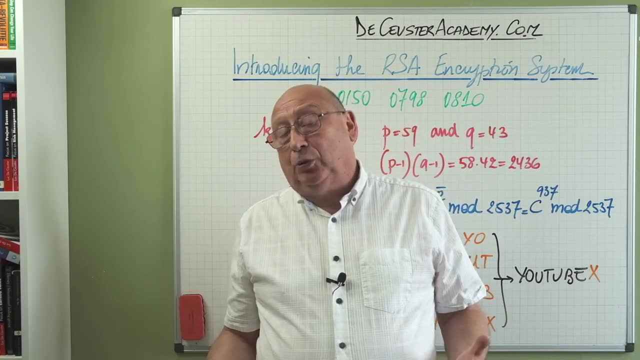 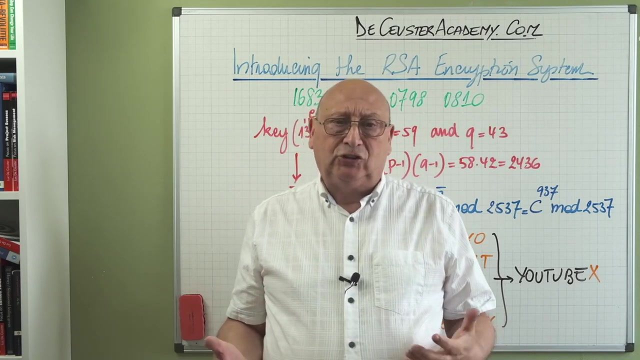 So that's the RSA encryption system: Basically unbreakable, But, like I said, new technologies evolve. Other possibilities are there. What will quantum computing do? It will be, or it can be, a game changer. We don't know yet, But there are some expectations that it will.